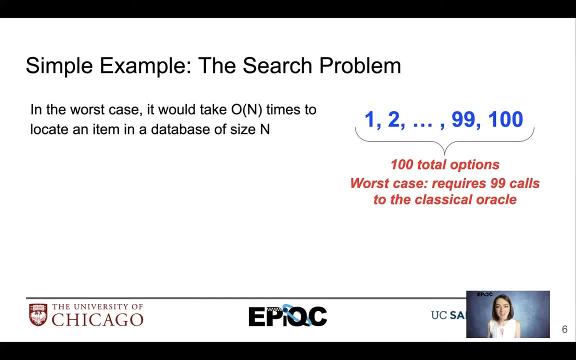 In the worst case, we would have to take big O to the N times to locate an item within this database of size N, with N being the number of items that we're searching through. If random access and presort were added to implement a binary search on ordered data, our search time would reduce. 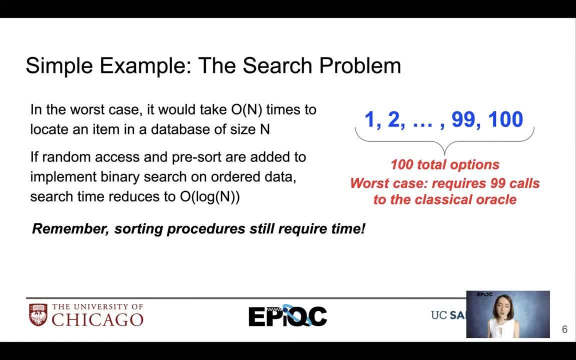 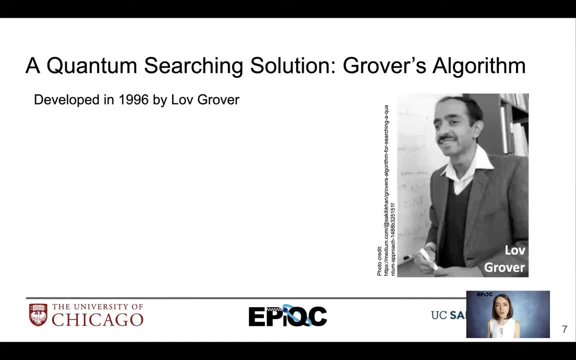 but these sorting procedures don't come for free. They still require some time to implement. So here we introduce a quantum solution: Grover's algorithm. Grover's algorithm was developed in 1996, and it is applicable to any problem that can be solved classically. 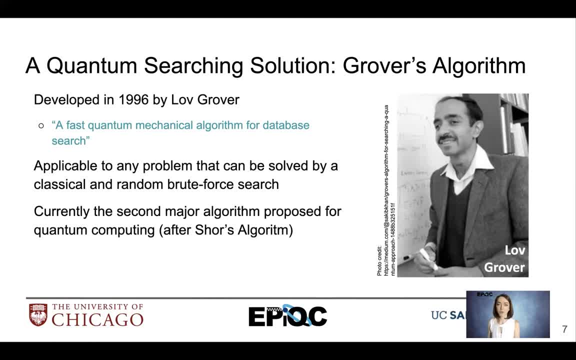 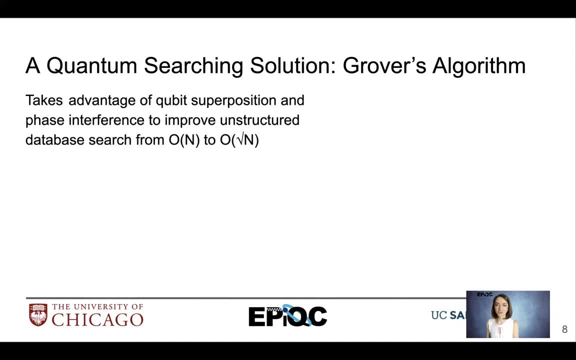 by a random brute first search. It's a major algorithm proposed for quantum computing and it's probably one of the most popular, right behind Shor's algorithm. So how does Grover's algorithm work? Grover's algorithm takes advantage of: 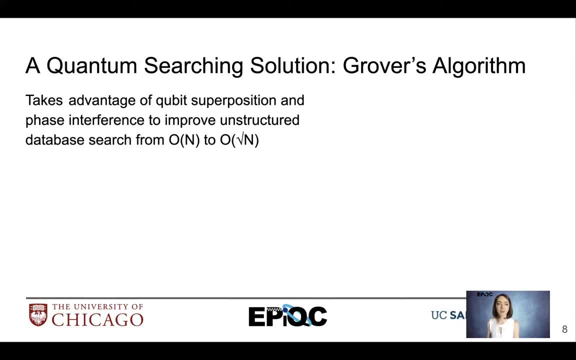 qubit superposition and phase interference to improve unstructured database search. from big O- n to big O square root of n. But what does that big O mean? Big O notation on a very high level means that it's the upper bound of the amount of time. 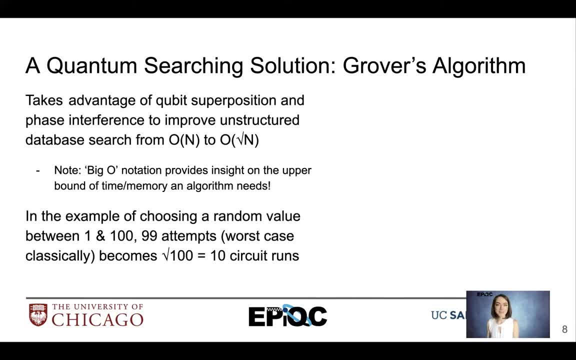 or memory that an algorithm needs to come up with a solution. So in the example of choosing a random number between one and 100,, 99 attempts at worst case classically would become square root of 100 or 10 circuit runs in the quantum case. 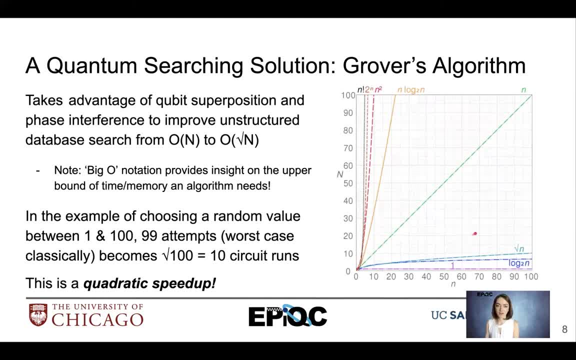 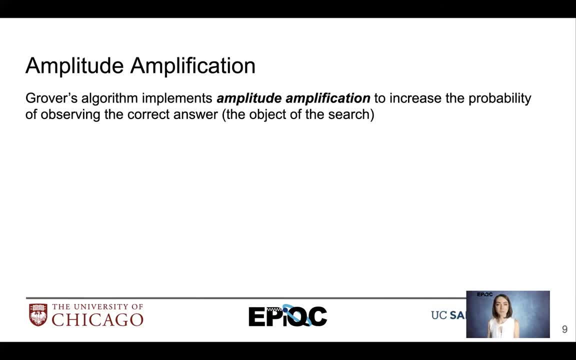 This is a quadratic speedup. We can look at this chart over here. we see that we have n reduced to square root of n. Amplitude amplification is one of the key components of Grover's algorithm that allows us to work. So what does this do? 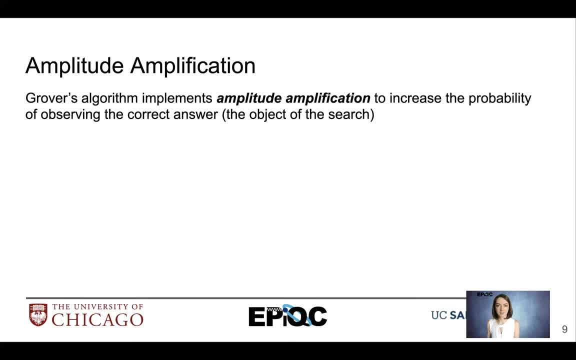 This allows us to increase the probability of observing the correct answer or the object of search. So we want to increase the probability amplitude associated with the answer ket, while simultaneously decreasing all other probability amplitudes. So if we have a balanced superposition and we're looking for a particular value, 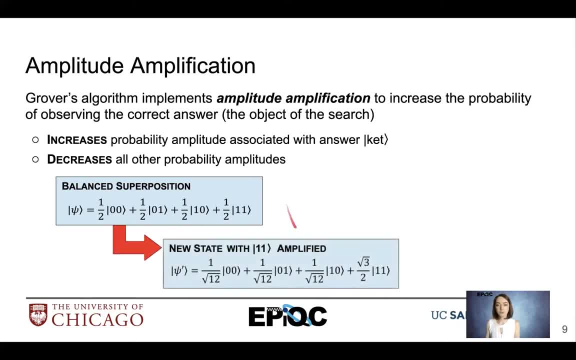 let's say ket one. we're going to boost ket one's probability amplitude while reducing all other basis ket probability amplitudes. And, as a note, we can see that the math checks out that all these probabilities will still sum to one that are associated with this state. 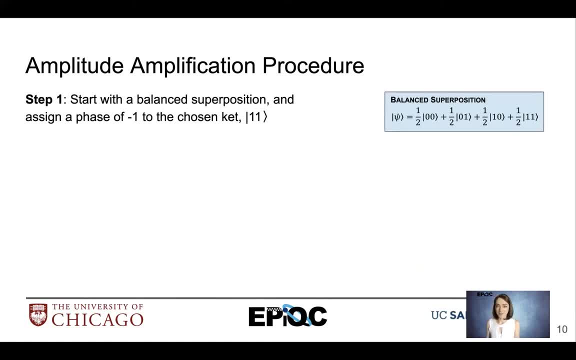 What is the procedure for amplitude amplification? We want to start with that balance superposition and we want to assign a phase of negative one to that chosen ket. So in our example, ket one one, So drawn out, we have our probability amplitude. 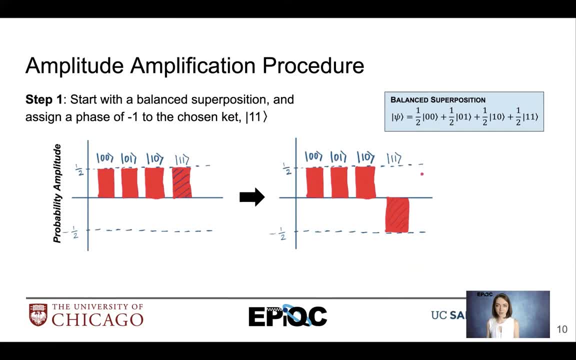 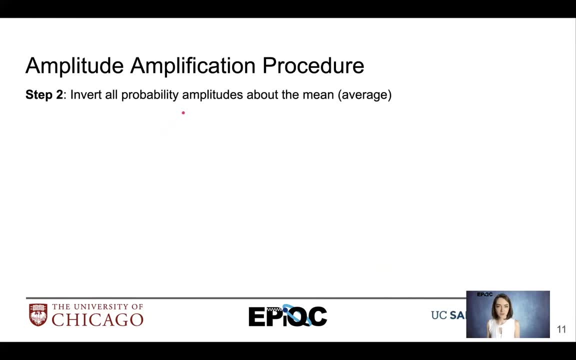 we're going to assign a negative phase to our chosen ket, so ket 1,1.. We're going to call the matrix that implements the phase flip u of f. Once we have our inverted phase, we're going to invert all amplitudes around the mean or average. So if we take the average of all of our probability, 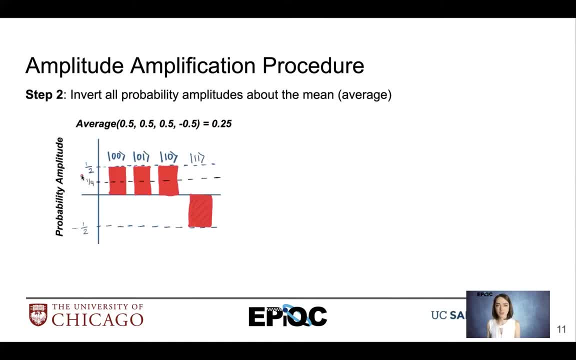 amplitudes, you'll get 0.25.. We have labeled 0.25 or one-fourth and we're going to invert all of our amplitudes around the mean. We see that all of our other kets go to 0, and our ket of search. 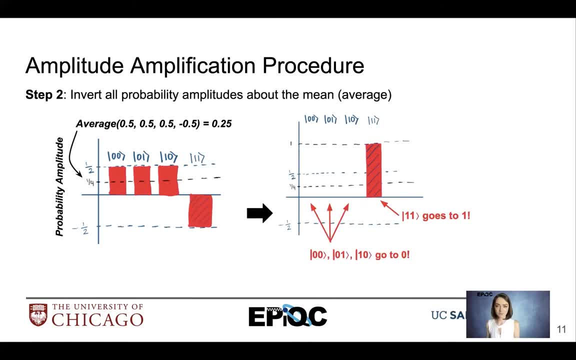 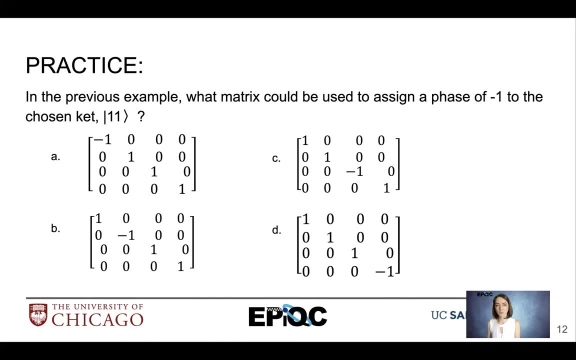 ket 1,1, goes to 1.. We will call the matrix that inverts around the mean u of phi. Let's take a second to do a little practice problem. In the previous example, what matrix could we use for that oracle that assigns phase of negative 1 to the chosen ket? It would be d, so we want to assign. 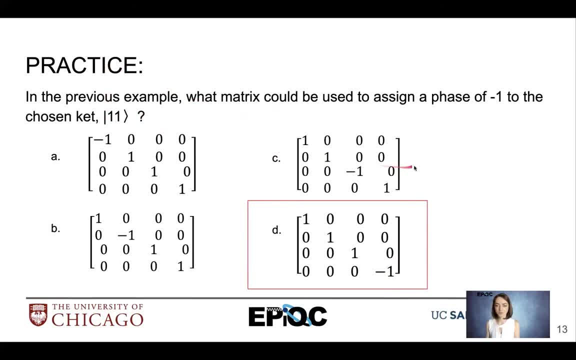 a negative 1 to the ket. We're going to call the matrix that inverts around the mean u of phi. We can try this out by multiplying this matrix with different two-qubit vectors. Amplitude amplification has two parts. There's the diffusion operation that inverts amplitudes. 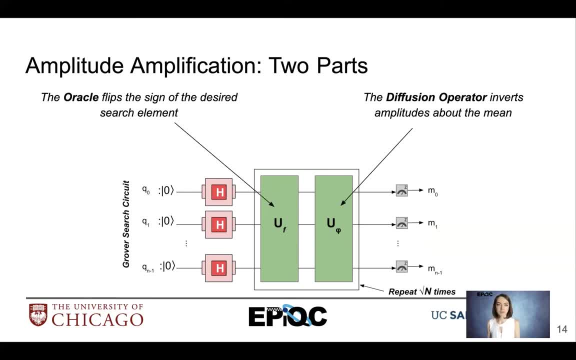 around the mean. and then there's the oracle that flips the sign of the desired search element so it assigns that phase of negative 1.. But there's a lingering question: How does the oracle know what to look for At a high level? what we're going to do is we're going to look at. 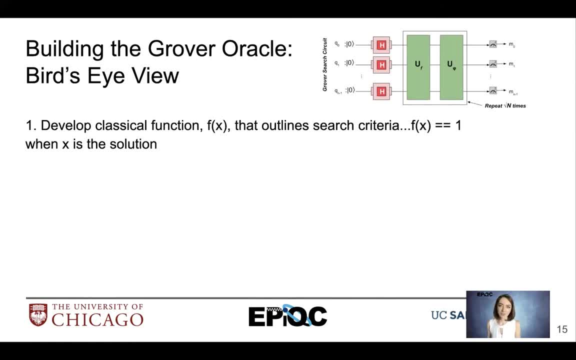 how to build this oracle. So we want to develop a classical function- We'll call this f of x- that outlines our search criteria. So f of x will equal 1 when x is the solution. We have to outline criteria such as: find an input x, that's a factor of 25, starting with these numbers, find an. 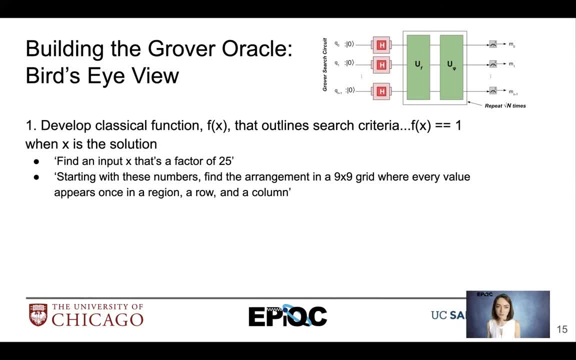 arrangement of a 9 by 9 grid where the Sudoku problem find the optimum route where I visit 300 stops only once. So we take all these and outline criteria. where f of x is the solution, f is equal to 0 if input x does not satisfy the criteria, but it's equal to 1 if x the input. 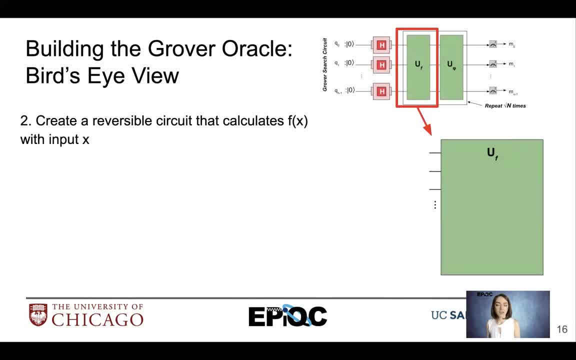 does satisfy the criteria. Next, we want to create a reversible circuit that calculates f of x with input x. Remember, we previously discussed how we can use different tools, like Ancilla, to create reversible functions out of irreversible functions. Once we have a reversible circuit generated, 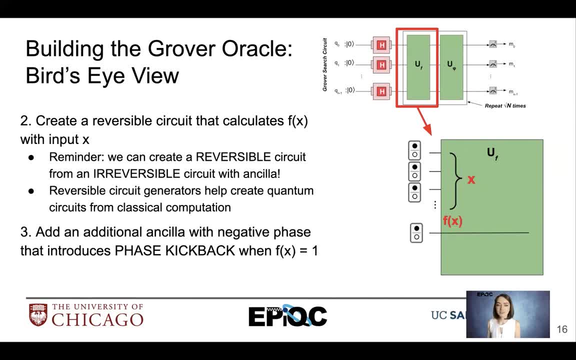 we add an additional Ancilla with negative phase that introduces phase kickback when f of x is equal to 1.. That allows our object of search to get a phase of negative 1.. So here we see our Ancilla with negative phase. If f of x is equal to 1, phase kickback occurs. Remember we learned about. 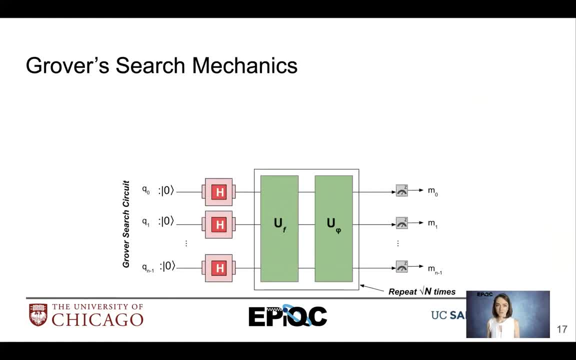 phase kickback in previous lectures. Now that we know how to construct the oracle, we're going to go ahead and create a new one. So we're going to create a new one. The first thing we're going to do is create an oracle and the main components of Grover's. 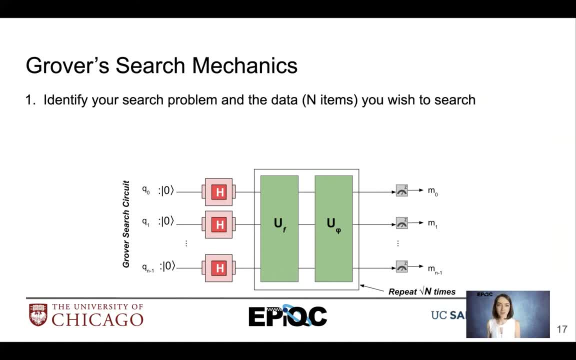 search. we'll talk about the mechanics. So we identify our search problem in the data, our n total items that we wish to search. Then we find the smallest number of n that satisfies n is less than or equal to 2. to the little n Our input, x will be representative of n qubits. 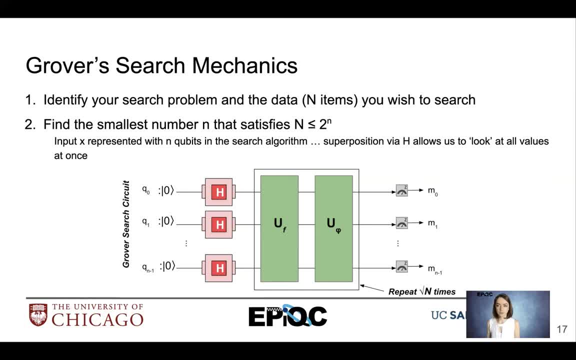 in the search algorithm and we'll put all those qubits into a superposition so we can look at all these values at once. We'll construct our oracle that will flip the sign of the object in search and our data will be represented in the search algorithm. So we'll need to find the n total. 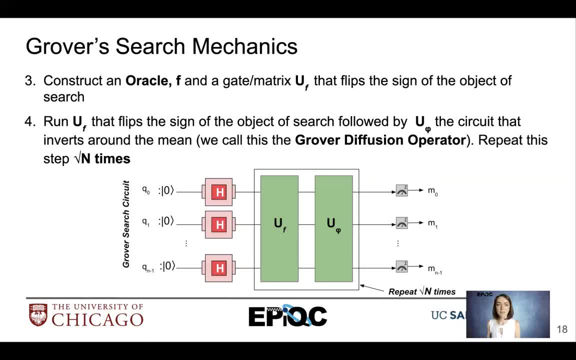 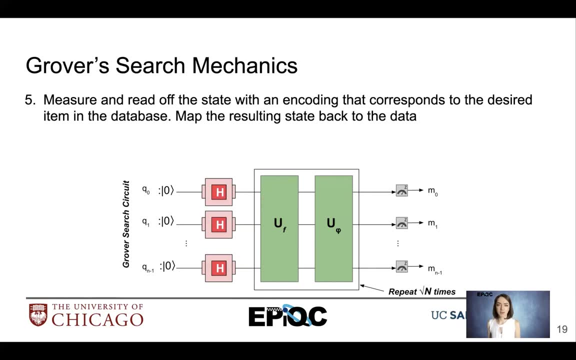 state u of f, that flips the sign of the object of search, and then we'll run u of f followed by u of phi, our Grover's diffusion operator, square root of n times. So we can see that here. Then we measure and read off the state with an encoding that corresponds to the desired. 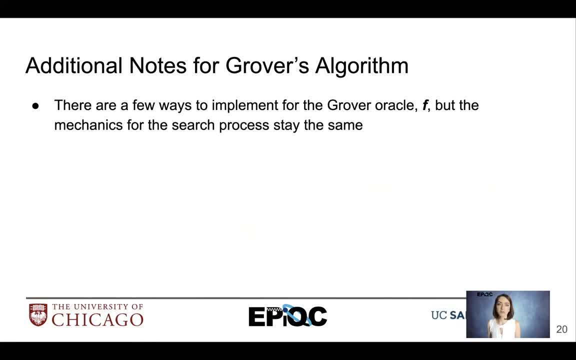 item in the database. Additional notes for Grover's algorithm include the following: There are a few ways to implement the Grover oracle f, but the mechanics for the search process stay the same. We searched for one item here, but there are variations of Grover's. 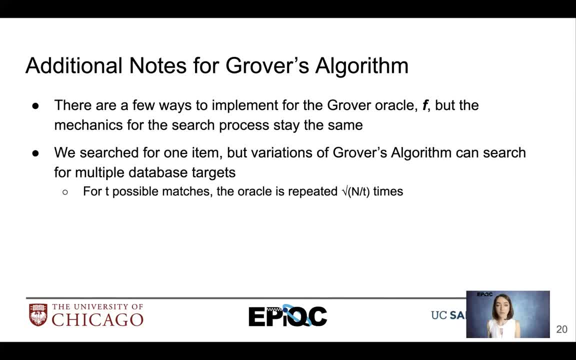 algorithm that can search for multiple database targets. So if we have the case where we're looking for t possible matches, the oracle is repeated: square root of n divided by t times. There's also the ability to do partial quantum search, So an example of this would: 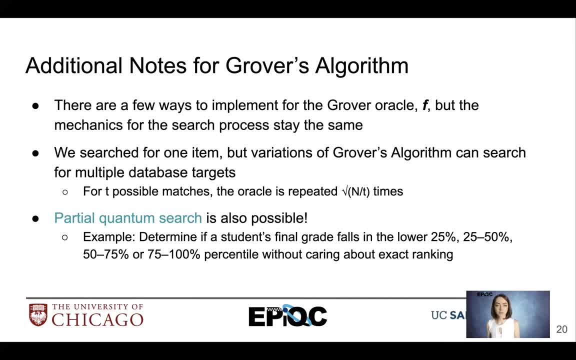 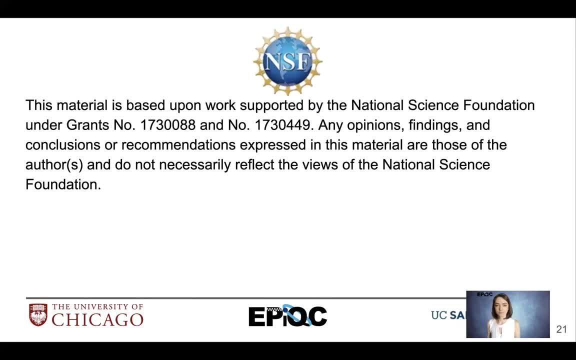 be determining if a student's final grade follows into a certain percentile without caring about the exact ranking of that student. Subtitles by the Amaraorg community. 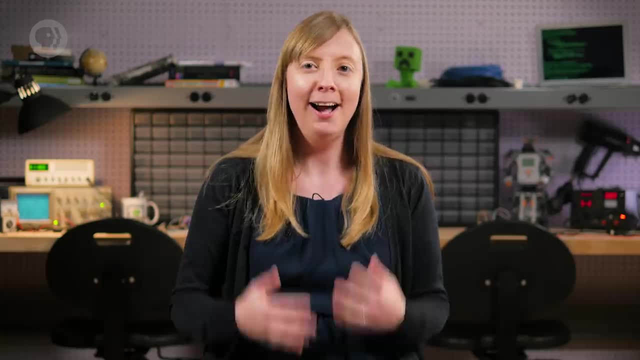 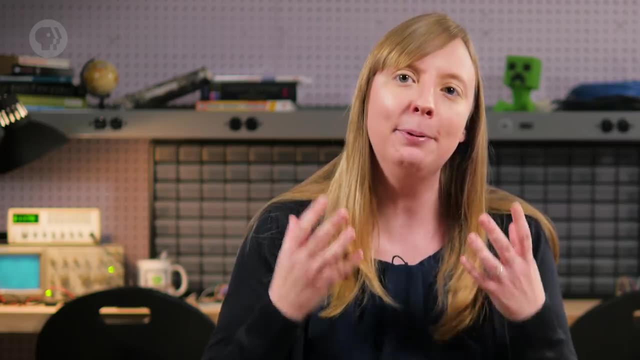 Hi, I'm Carrie-Anne and welcome to Crash Course Computer Science. Today we start our journey up the ladder of abstraction, where we leave behind the simplicity of being able to see every switch and gear but gain the ability to assemble increasingly complex systems. 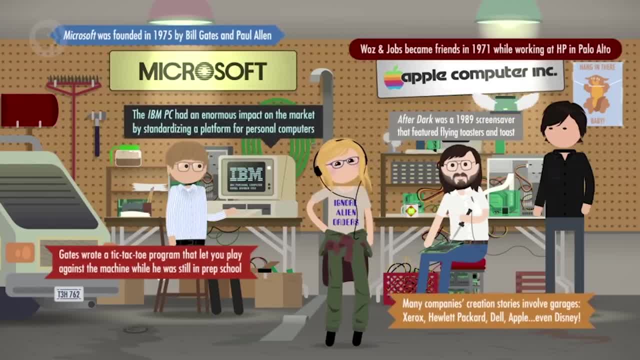 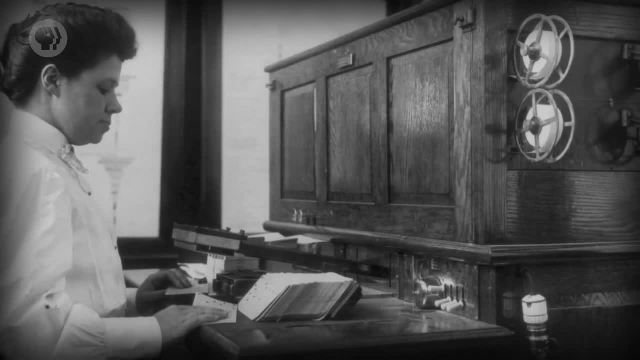 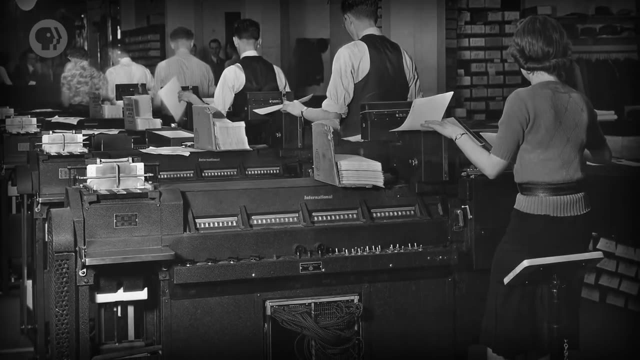 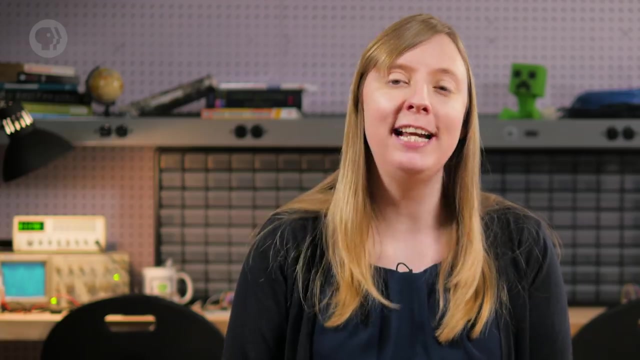 Last episode we talked about how computers evolved: from electromechanical devices that often had decimal representations of numbers, like those represented by teeth on a gear, to electronic computers with transistors that can turn the flow of electricity on or off. Unfortunately, even with just two states of electricity we can represent important information. 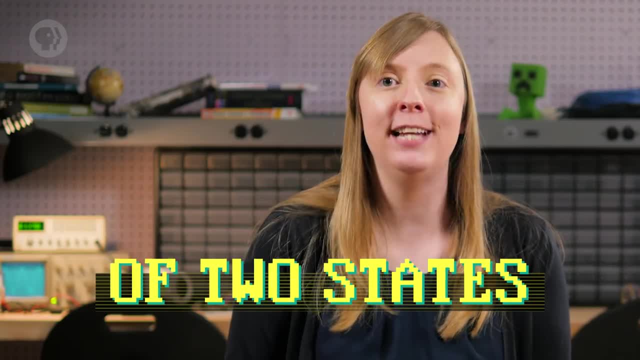 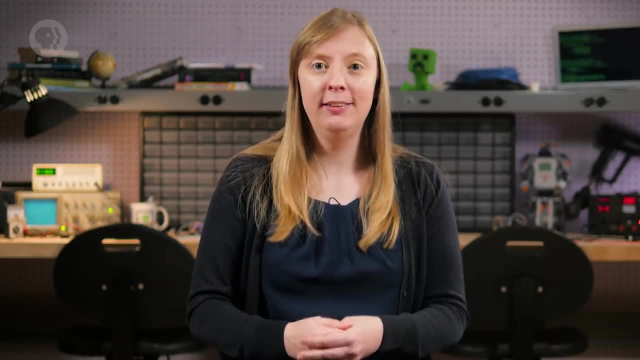 We call this representation binary, Which literally means of two states. in the same way, a bicycle has two wheels or a biped has two legs. You might think two states isn't a lot to work with, and you'd be right, but it's. 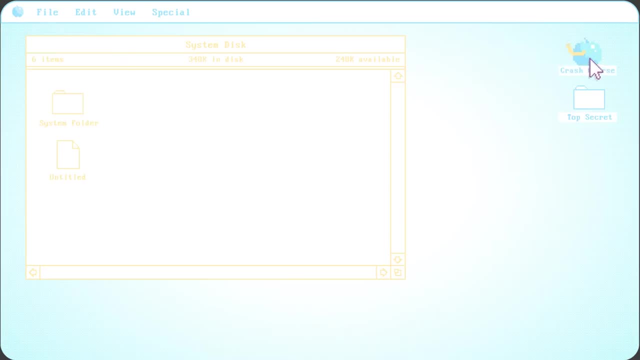 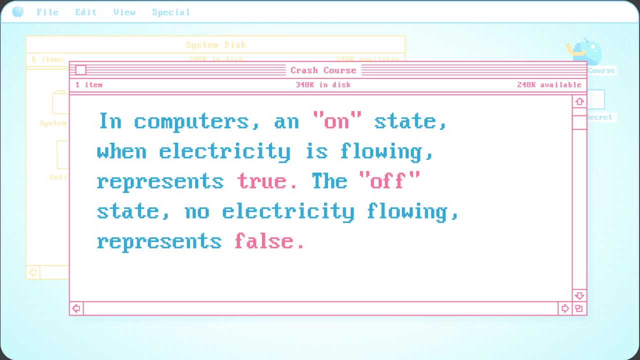 exactly what you need for representing the values true and false In computers. an on state when electricity is flowing represents true. The off state, no electricity flowing, represents false. We can also write binary as ones and zeros instead of trues and falses. 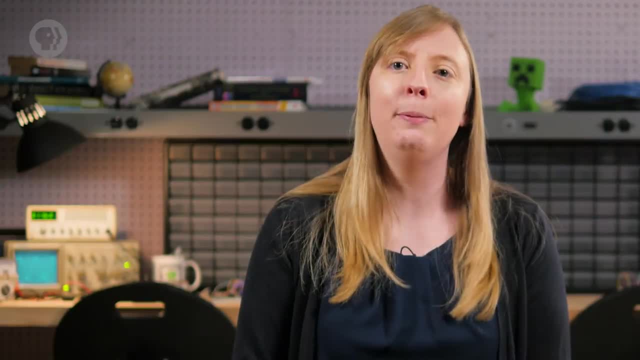 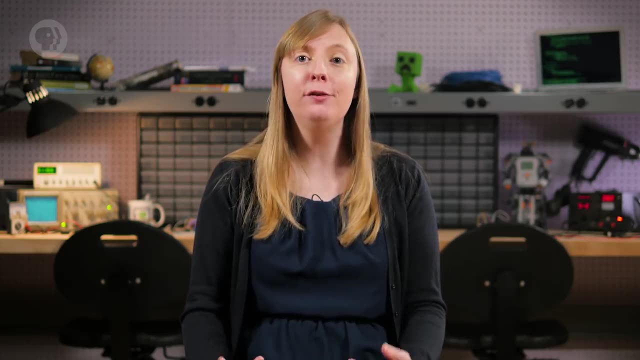 They are just different expressions of the same signal, But we'll talk about that in the next episode. Now it is actually possible. It's even possible to use transistors for more than just turning electrical current on and off and to allow for different levels of current.